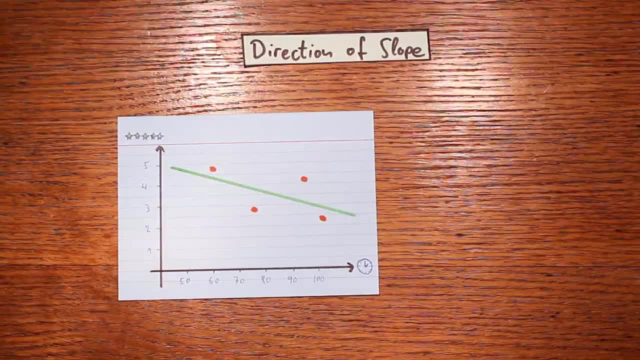 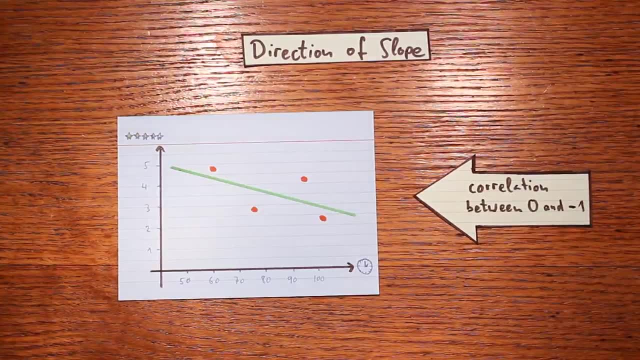 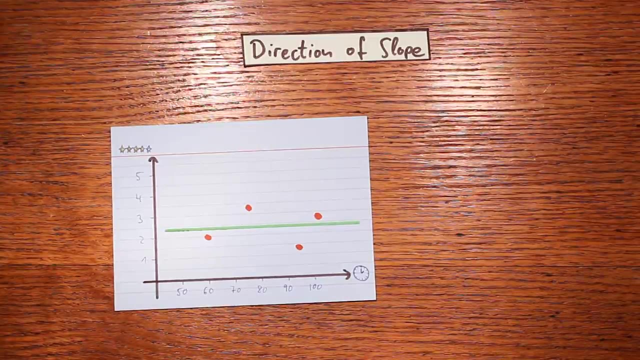 the longer movies tend to get the worst ratings. so the slope is negative, And in that case the correlation coefficient is negative as well. It'll be between 0 and minus 1.. And then there's a third case, and that's that the slope is perfectly straight. In this data set you can see that 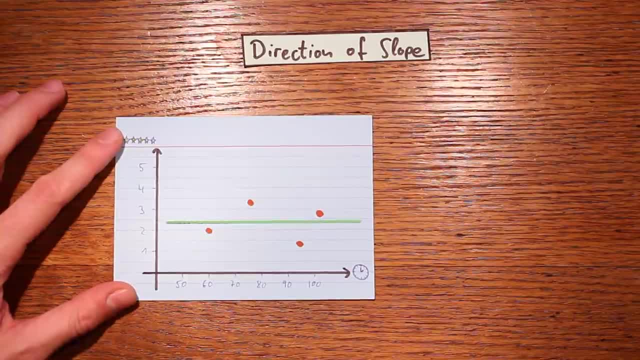 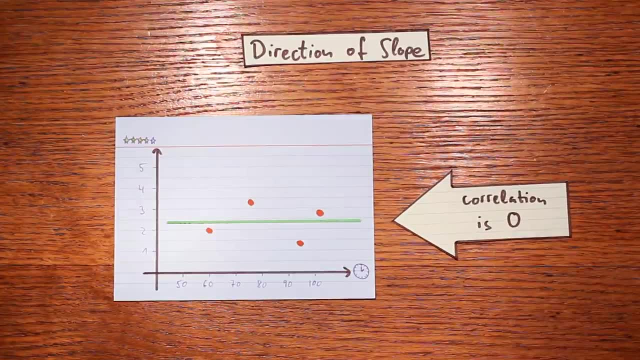 there's no real difference between the longer and the shorter movies in terms of rating And actually if I draw in the regression line, you can see that it's perfectly straight And in that case the correlation coefficient is 0.. So just by looking at the sign of the correlation, you 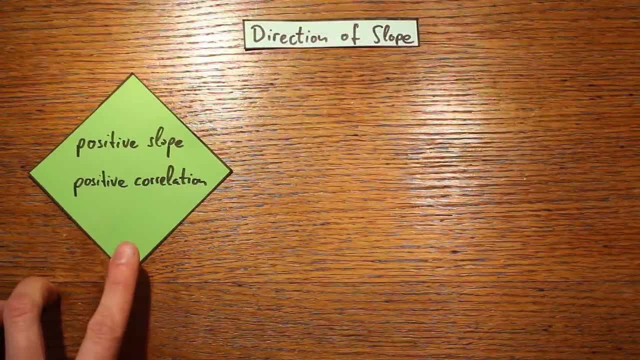 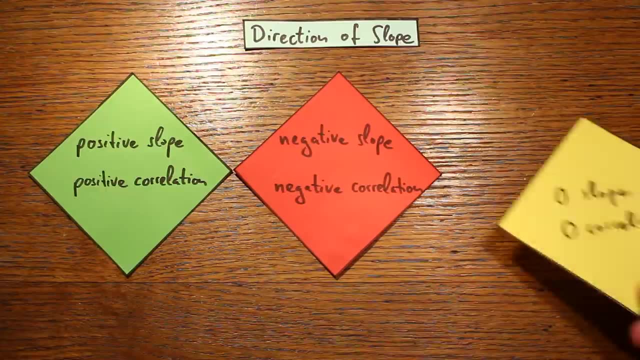 already know something about your data. If the correlation is positive, you know that the overall trend is upwards. If the correlation is negative, you know that the overall trend is downwards. And if the correlation is 0, you know that the overall trend is level. So now comes the third step, but this one is: 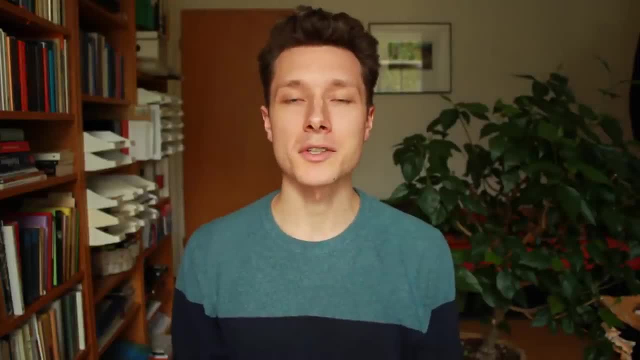 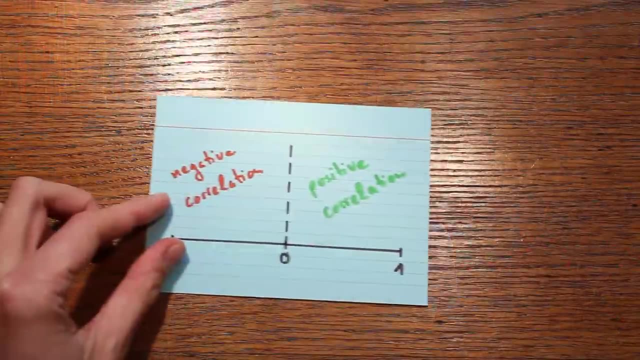 trickier. So so far we already know whether the correlation coefficient is between 0 and 1, or 0 and minus 1. But we don't know its magnitude yet. So how big is the value? Is it close to the? 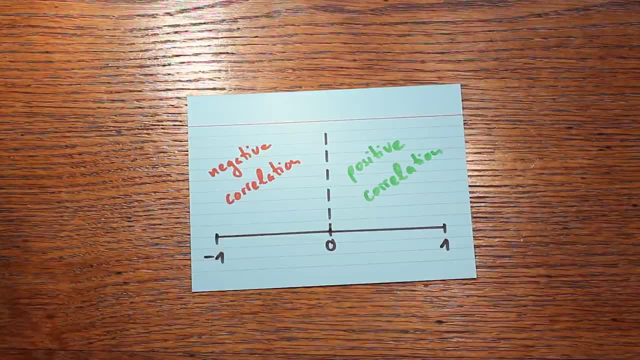 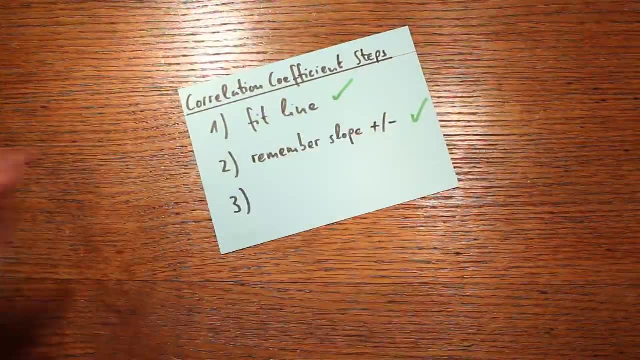 extreme value, so something like 0.92 or minus 0.92? Or is it small in magnitude because the correlation is weak, so it's closer to 0?? The correlation coefficient figures this out by looking at the quality of the correlation coefficient. So if the correlation coefficient 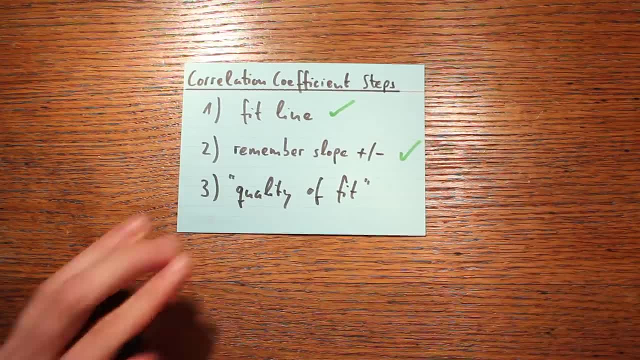 is 0,, they are closer to 0.92 and minus 1.92, and if the correlation coefficient is 0, it's something like 0.02.. So the correlation coefficient figures this out by looking at the quality of the correlation. 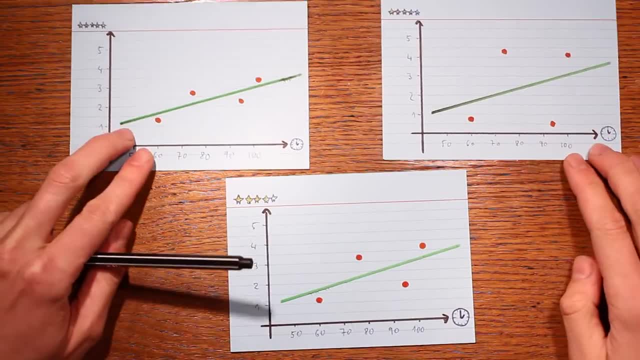 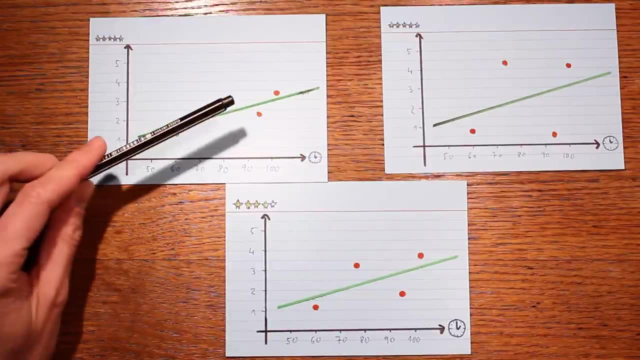 coefficient. So what do we come up with? We come up with a first-year, initial phase of the correlation coefficient, which is the cost of the correlation coefficient, which is the cost of the correlation coefficient and the past ratio, the cost of the correlation coefficient. We then 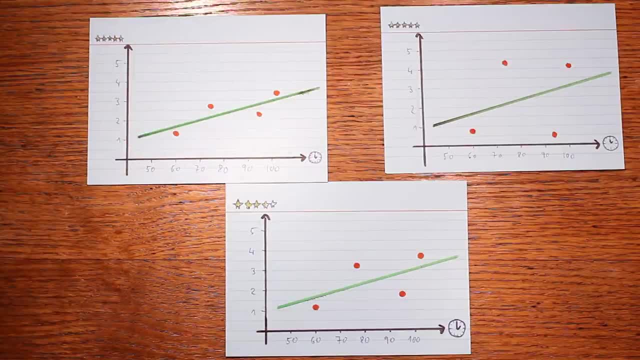 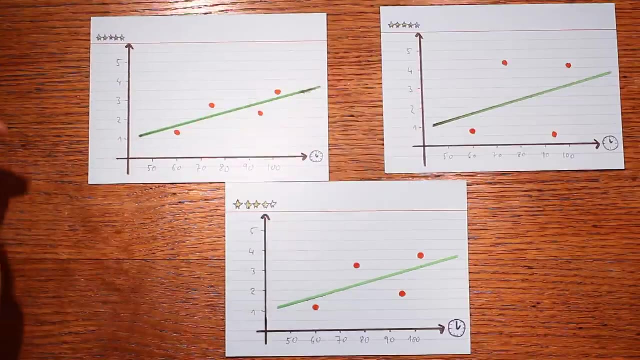 jump into that. Here's an example of the fit of this straight line for the data and I'll try to give you three plots. the highest correlation would be in this plot and the lowest correlation would be in this plot. Actually, the correlation coefficient for the first plot is around 0.81,. 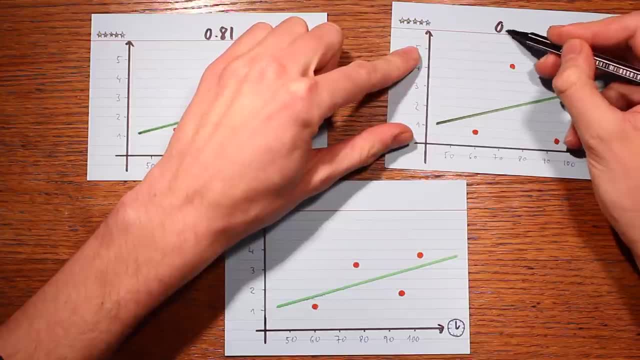 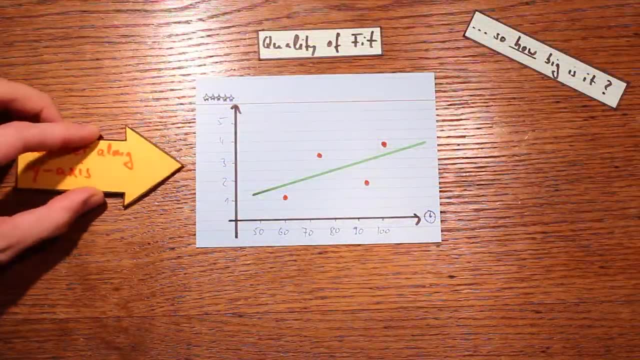 and the correlation coefficient for the worst plot is 0.32, so it's much lower. But how does the correlation coefficient figure this out? Well, it compares two things. The first thing it looks at is the scatter along the y-axis. So if I draw in the y-values, 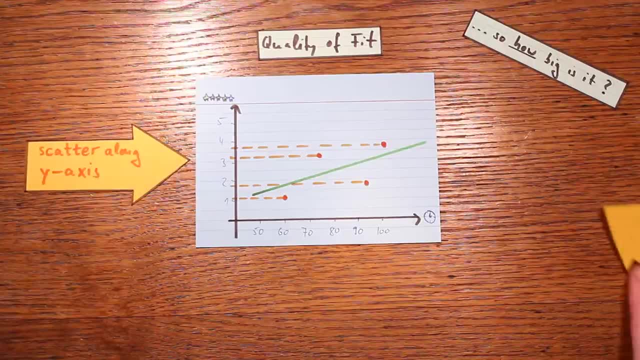 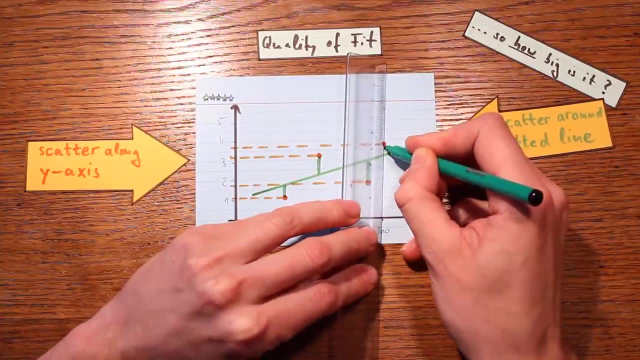 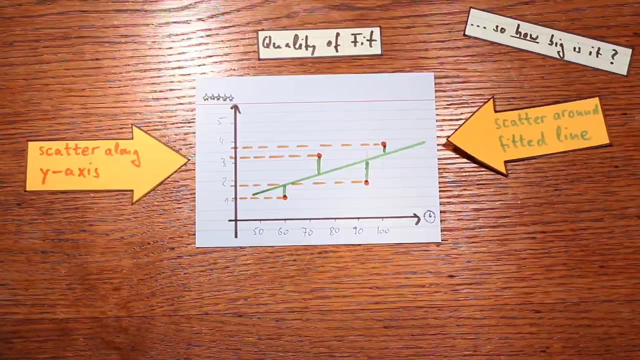 you can see how they scatter along the y-axis. The second thing it looks at is the scatter of the data around the fitted line, So that corresponds to these distances here, And the rule goes like this: The more there's of this in comparison to this, the stronger the correlation. 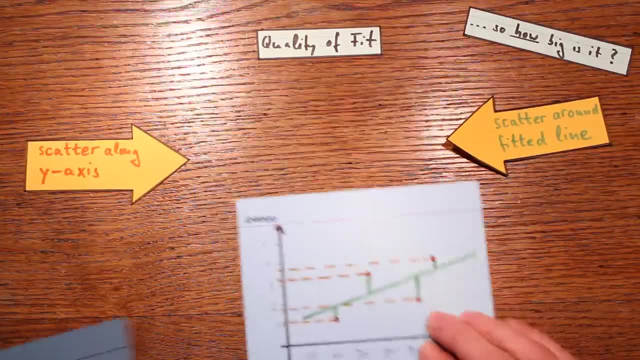 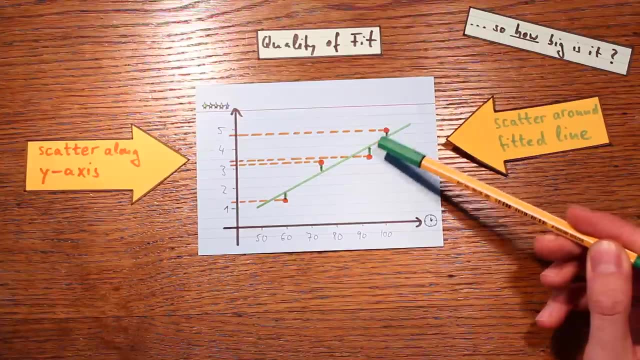 coefficient is Okay. let me show you a few examples. So in this dataset we can see that there's quite a lot of scatter along the y-axis, but there's really little scatter around the fitted line right, Because the distances here 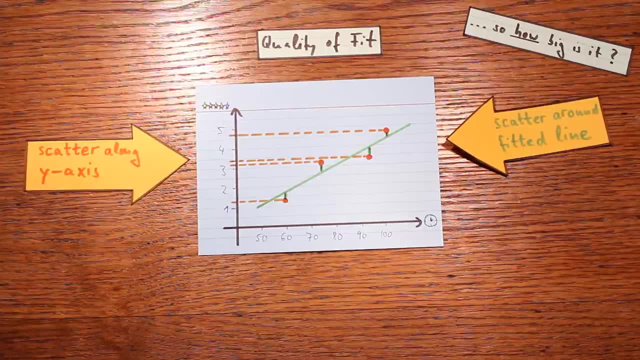 of the data points from the fitted line. they are really short, Okay. so in comparison there's a lot more scatter along the y-axis than there's scatter around the fitted line, And in this case the correlation coefficient is really large in magnitude. This is a positive 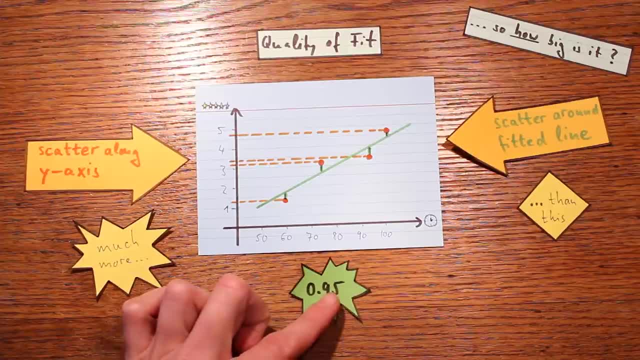 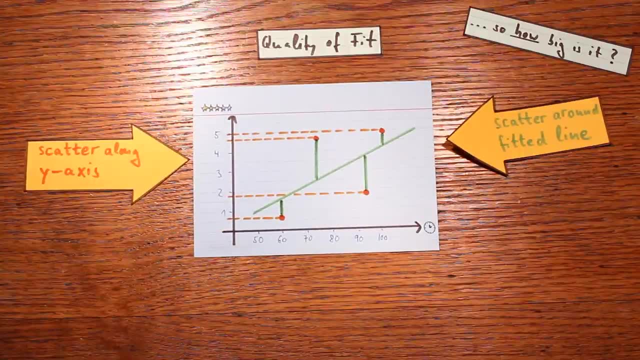 slope. so the correlation coefficient is close to 1.. It's actually 0.95, so that's a really strong correlation. And here's a second case. So you can see that again we have quite some scatter along the y-axis, but in this example the scatter around the fitted line 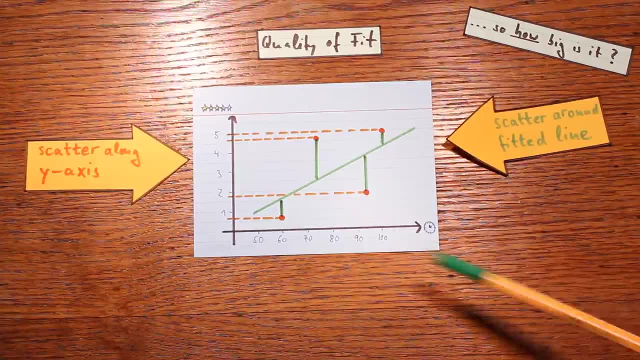 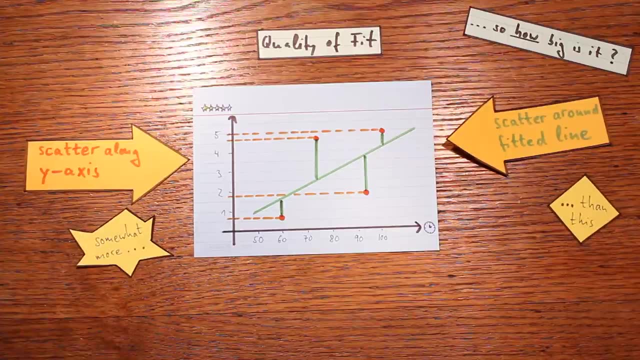 is also really large, right, The points are really far away from the fitted line. Okay. so in comparison, there's only somewhat more scatter along the y-axis than there's scatter along the fitted line. So in this case the correlation coefficient is weaker: It's 0.56,. 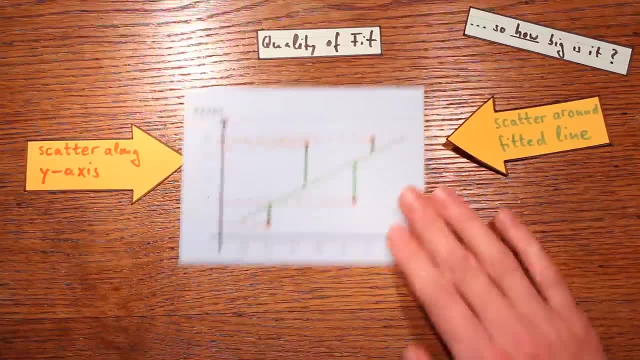 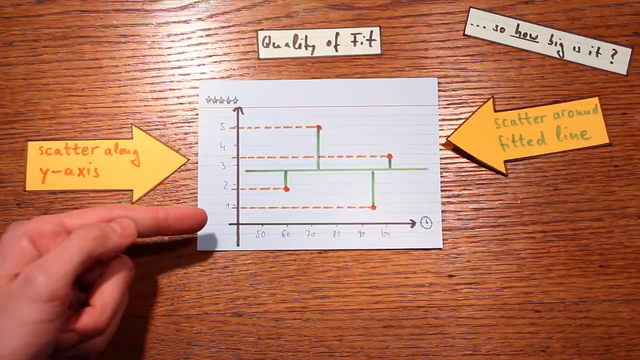 actually, That's still decent correlation, but it's less than before. In this third case, the fitted line actually turns out to be straight. So what this means for the data is that the scatter along the y-axis and the scatter around the fitted line 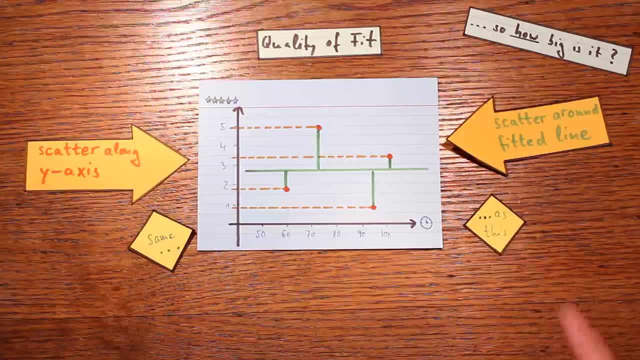 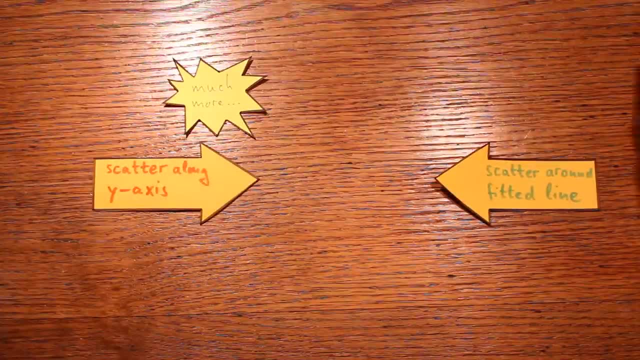 are actually exactly equal And in this case the correlation coefficient is exactly 0.. So you can see that if the scatter along the y-axis is much larger than the scatter around the fitted line, then we get correlation coefficients which are really large in magnitude. But if